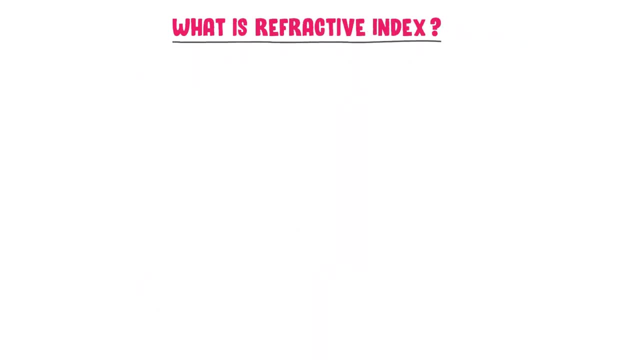 What is refractive index? Well, consider that an incident light ray is traveling in the vacuum. Let it hits the surface of a glass and enter into it. We know that light is refracted towards the normal. in this case, The speed of light in the vacuum is 3 into 10 to the power, 8 meter per. 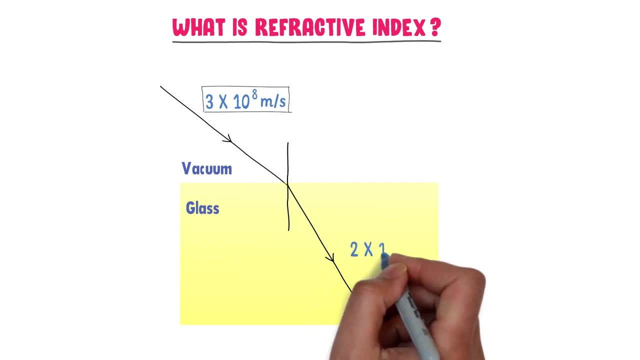 second, while the speed of light in the glass is 2 into 10 to the power, 8 meter per second. So we say that the speed of light in the vacuum is high and the speed of light in the glass is slow. Now, if I ask you why the speed of light is high in the vacuum and slow in the glass, then the answer is simple. It is because the vacuum is optically rarer medium. it means that vacuum shows less resistance to the speed of light, While glass is optically denser medium. it means that glass shows more resistance to the speed of light. 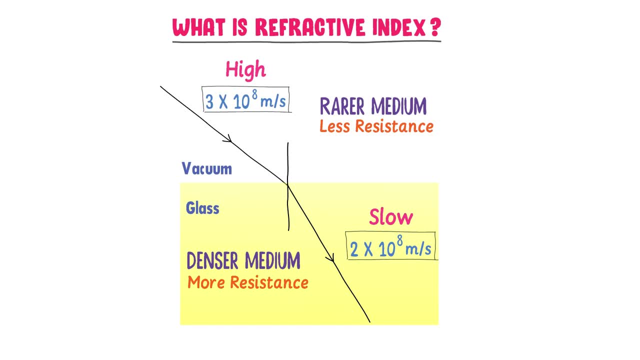 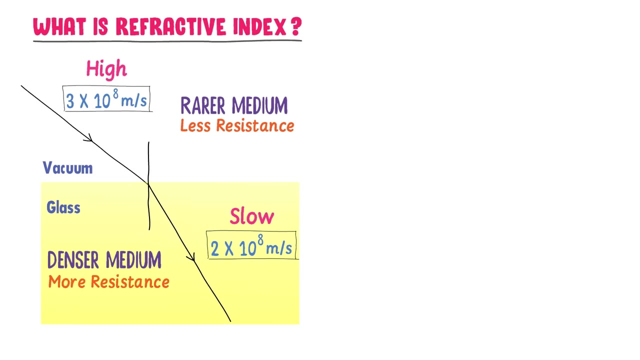 Thus, the first fact is that if a medium is less optically denser, speed of light is high. The second fact is that if a medium is more optically denser, speed of light is slow. Now listen carefully How we can measure optical density of a medium. 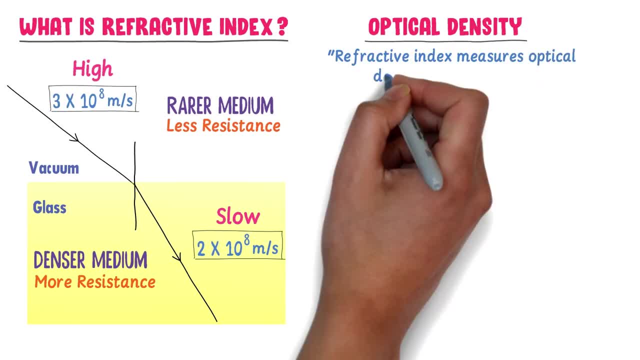 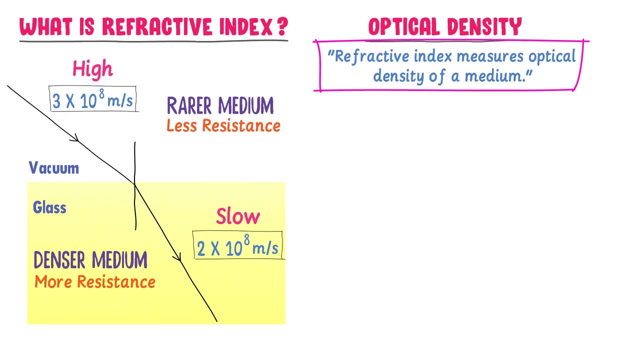 Well, refractive index measures the optical density of a medium. Let me repeat: Refractive index measures the optical density of a medium, wall density of a medium. So refractive index is nothing but the optical density of a medium. For example, I am interested to find that how much speed of light slows down in glass? 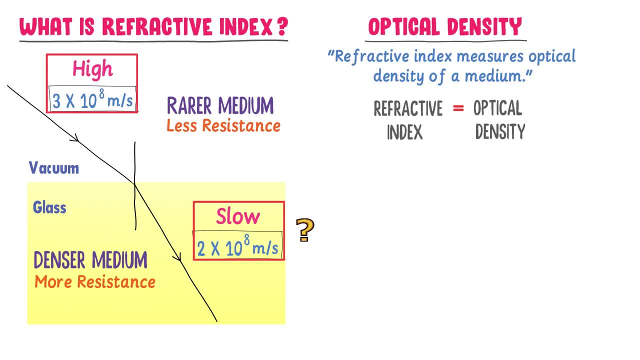 with respect to vacuum. So I will find the ratio of speed of light in a vacuum to the speed of light in a glass, For instance, speed of light in a vacuum upon speed of light in a glass. We know that the speed of light in a vacuum is 3 into 10 to the power 8 meter. 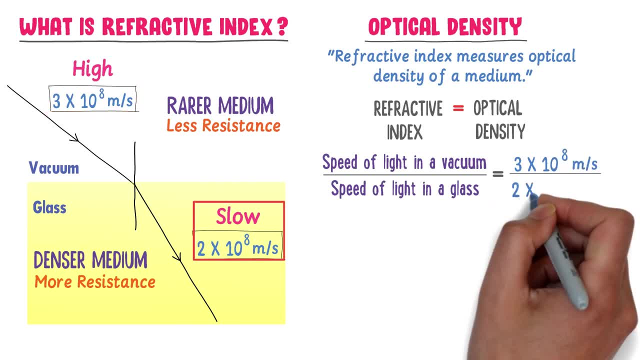 per second and the speed of light in a glass is 2 into 10 to the power, 8 meter per second. After calculation I get 1.5.. What does this 1.5 mean? Firstly, it shows the optical density. 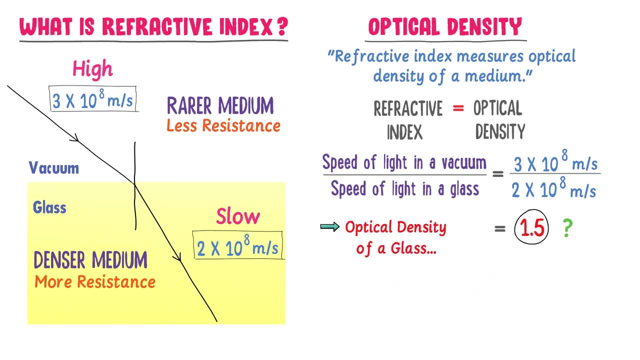 of a glass relative to vacuum. Secondly, it shows that speed of light is 1.5 times slower in glass than vacuum. Let me repeat this important point: It shows that speed of light is 1.5 times slower in glass than vacuum. Hence we therefore say that optical density. 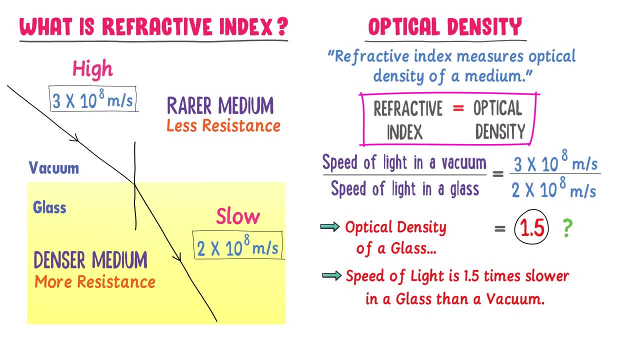 and refractive index are same thing, are two faces of same coin. So this 1.5 is also called reflective index of the glass. Therefore we define refractive index as the ratio of the speed of light to the speed of light, For instance, Infrared with glasses. it comes. 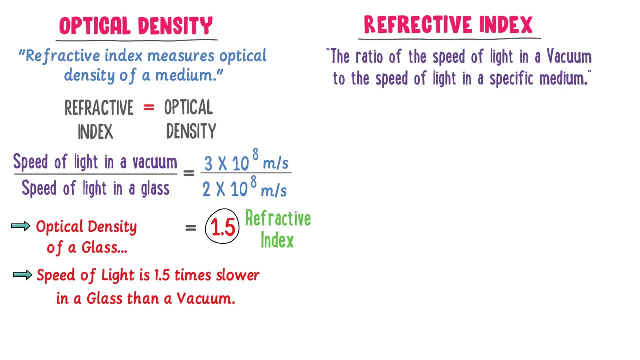 1.5 times slower in glassang vacuum. Let me repeat this important point. It shows that light in a vacuum to the speed of light in a specific medium is called refractive index. It is denoted by n. Mathematically we write: refractive index is equal to speed of light. 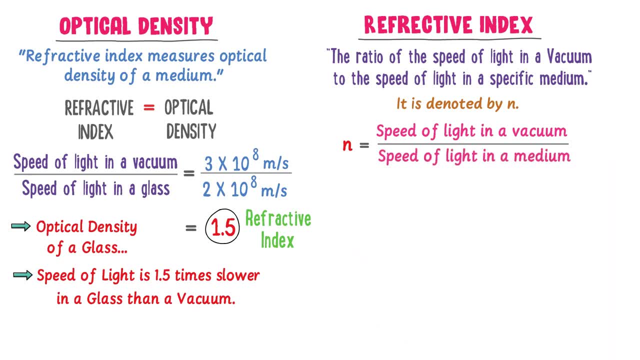 in a vacuum upon speed of light in a specific medium, or n is equal to c upon v, where c is the speed of light in a vacuum, which is a constant value, and v is the speed of light in a specific medium like glass, water, etc. Remember that this refractive index is also 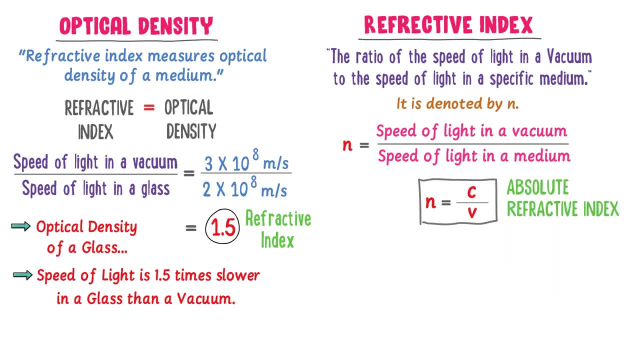 called absolute refractive index. Also noted down that when refractive index n is greater, medium is more optically denser and speed of light and it will be slow. Secondly, when refractive index n is smaller, medium is less optically denser and speed of light and it. 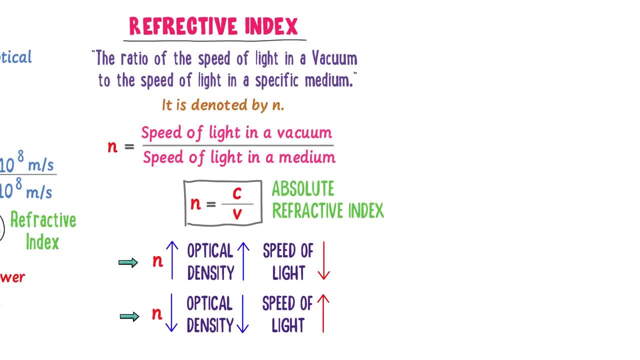 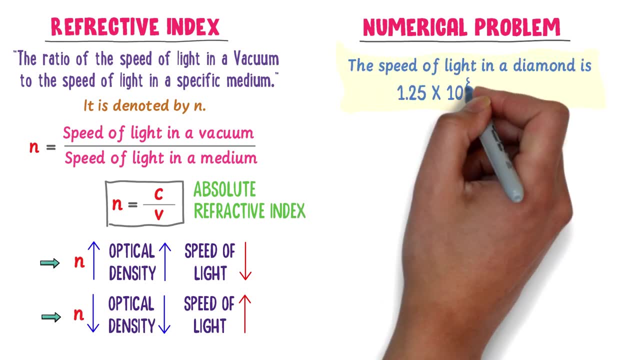 will be high. Now let me teach you that how to write refractive index. For example, the speed of light in a diamond is 1.25 x 10⁸ m per second. Find its absolute refractive index. Firstly, let me draw a freehand diagram so that you could. 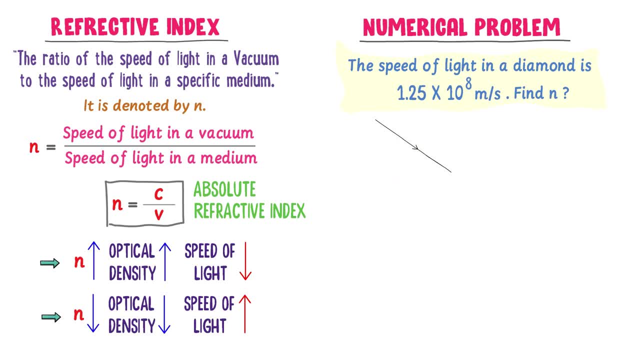 easily understand it. Let the incident. light ray is traveling from the vacuum and entering into the diamond. We know that the speed of light in the vacuum is: c is equal to 3 x 10⁸ m per second, and the speed of light in the diamond is given. 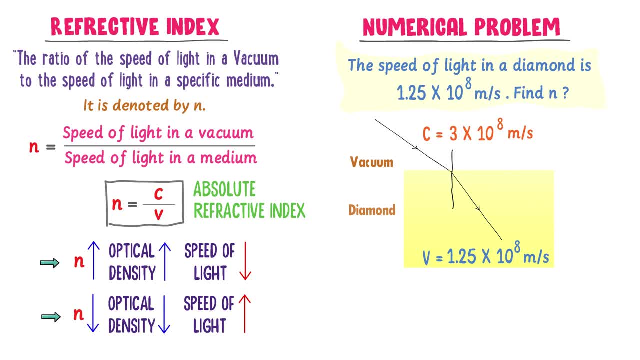 v is equal to 1.25 x 10⁸ m per second. As we learned in the previous slide that refractive index n is equal to c upon v, where c is the speed of light in the vacuum and v is the speed of light in the medium, like diamond. 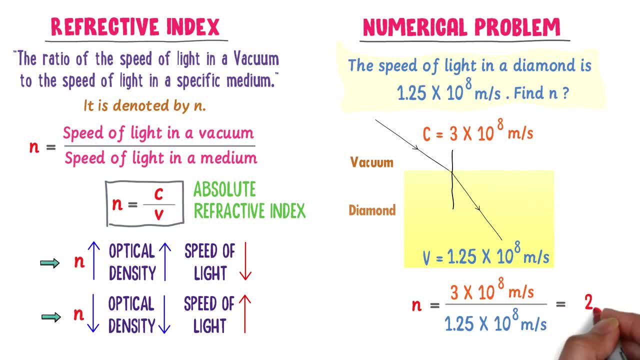 So we can easily find the absolute refractive index in this equation. After calculation I get 2.4.. So the refractive index of the diamond is 2.4.. What this 2.4 refractive index of the diamond means? Well, it means that the speed of light is 2.4 times slower in. 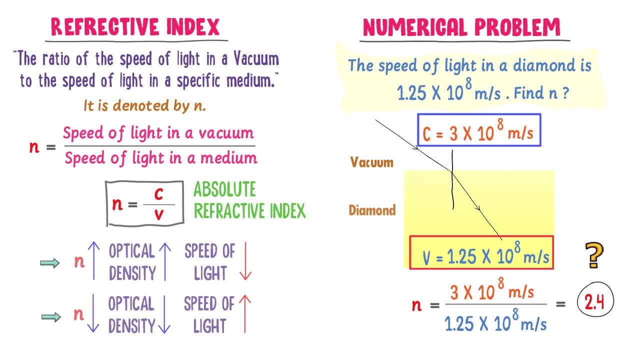 the diamond than the speed of light in the vacuum. Thus, by this way we can easily find the absolute refractive index of any medium. Here let me teach you 2.4 x 10⁸ m per second. Let me teach you two bonus MCQs Refractive index is unitless or it has no unit, If you. 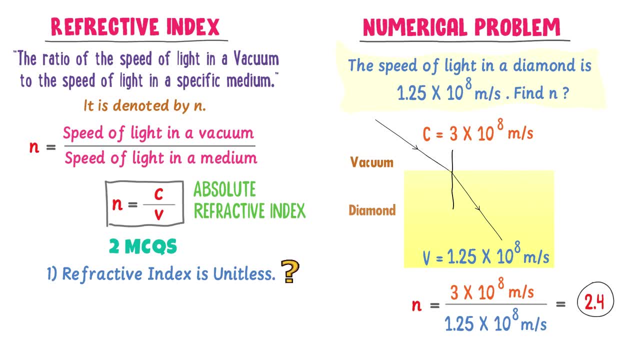 ask me why then? it is because refractive index is a ratio between two similar quantities, For example the unit of speed and numerator and the unit of speed and denominator. cancel out. We therefore say that refractive index is unitless or having no unit. Secondly, absolute. 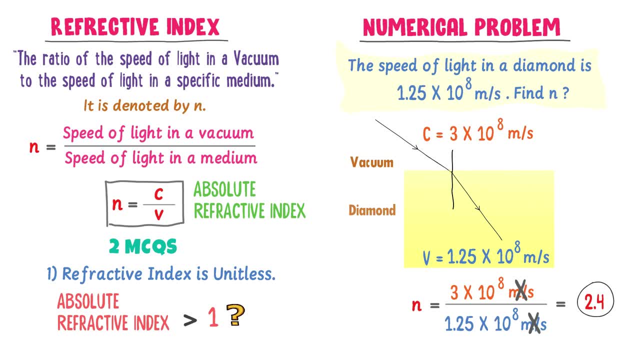 index is always greater than 1.. If you ask me why, then it is because in case of absolute refractive index, light always travel from the vacuum, a rarer medium, and to denser medium like glass. So the speed of light always slow down in the denser medium and absolute refractive index. 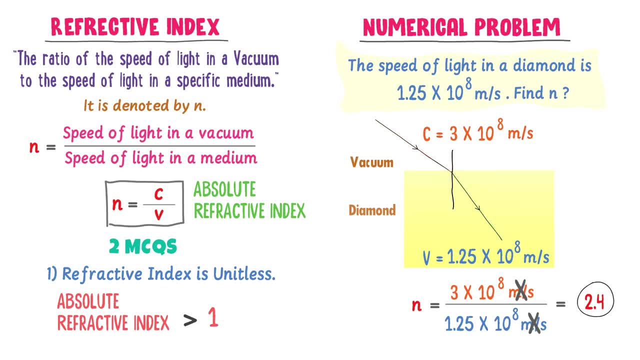 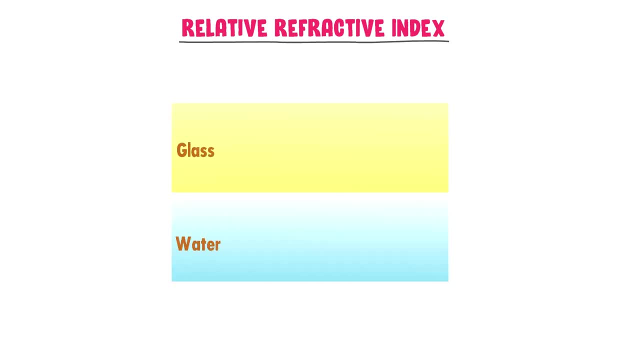 is therefore always greater than 1.. Finally, let me quickly teach you the concept of relative refractive index. Let consider a glass and water. Let an incident light ray is traveling from the glass and to the water, So it is refracted away from the normal. in this case, Let glass is first. 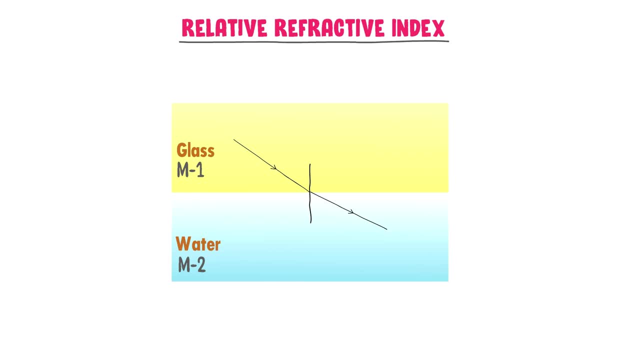 medium and water is second medium. The speed of light in the glass is 2 and to 10, to the power 8 meter per second, while the speed of light in the water is 2.25 and to 10 to the power, 8 meter.